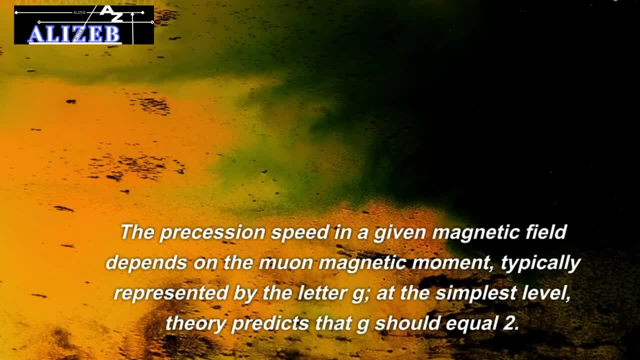 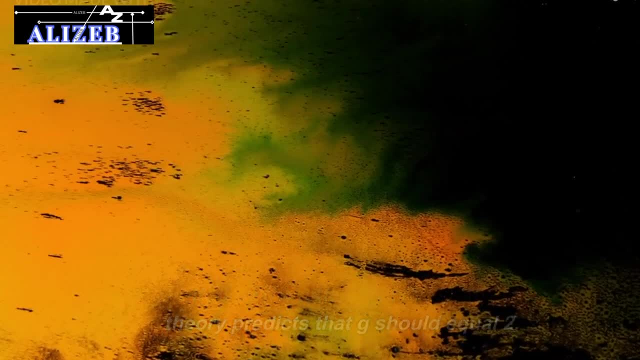 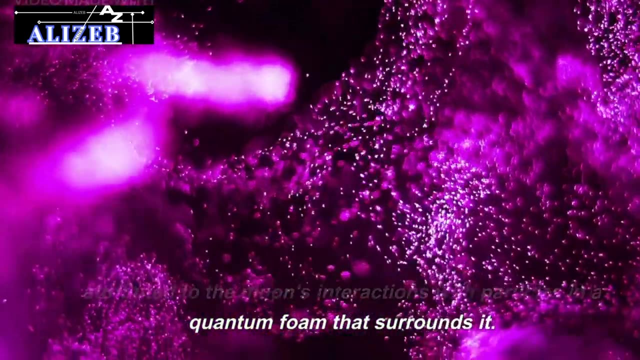 The precession speed in a given magnetic field depends on the muon magnetic moment, typically represented by the letter G. At the simplest level, theory predicts that G should equal 2.. The difference of G from 2 or G minus 2 can be attributed to the muon's interactions with particles in a quantum. 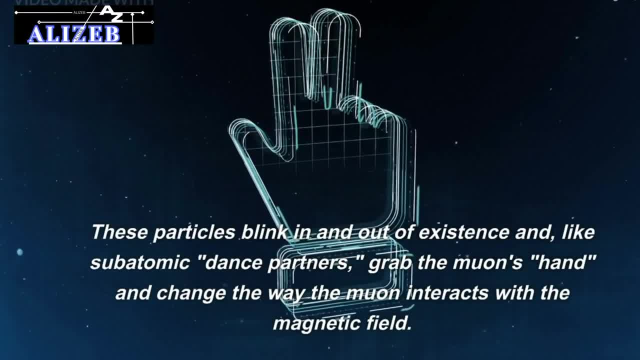 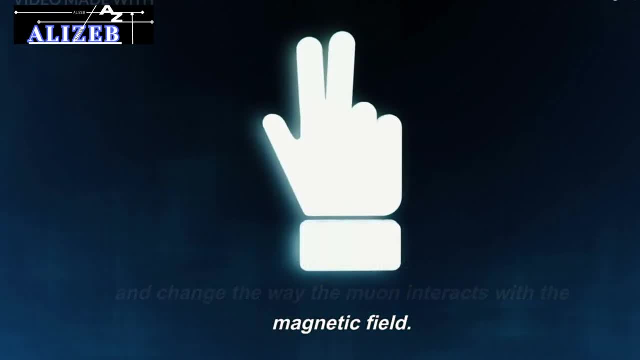 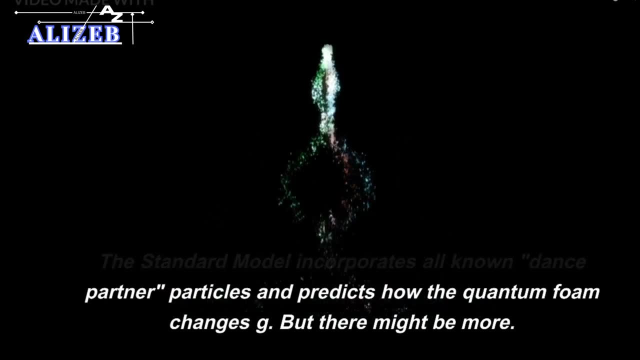 foam that surrounds it. These particles blink in and out of existence and, like subatomic dance partners, grab the muon's hand and change the way the muon interacts with the magnetic field. The standard model incorporates all known particles and predicts how the quantum foam changes. G, but there might be more. 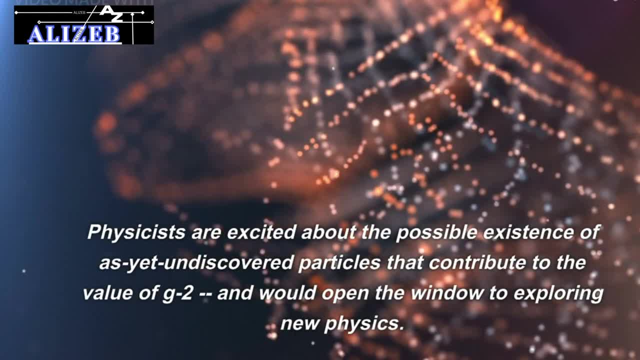 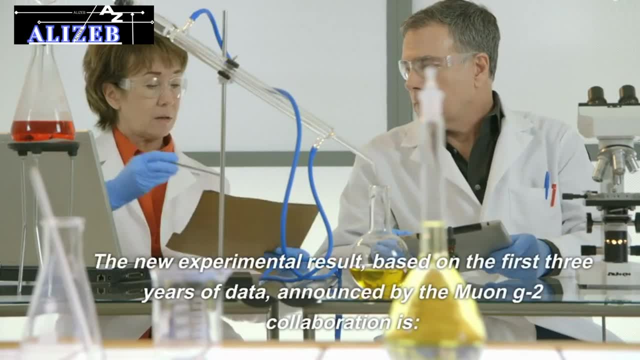 Physicists are excited about the possible existence of as-yet-undiscovered particles that contribute to the value of G2 and would open the window to exploring new physics. The new experimental result based on the first three years of data announced by the muon-G2 collaboration is: 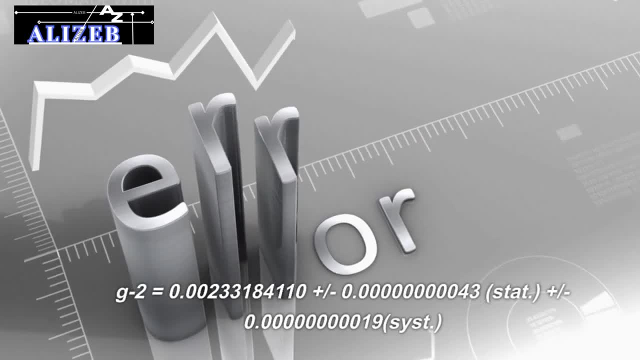 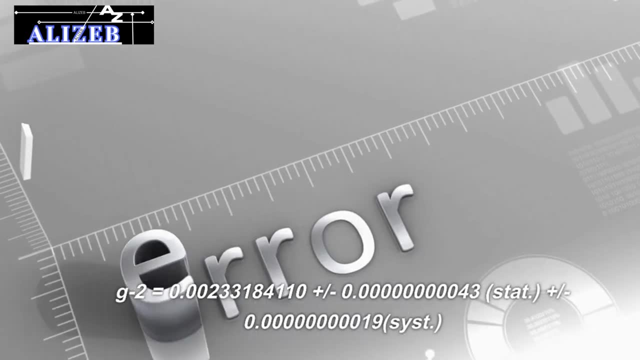 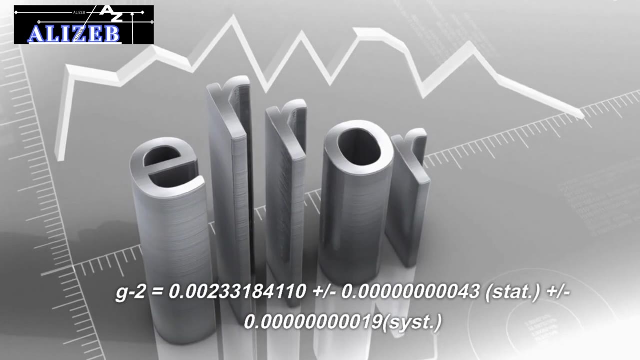 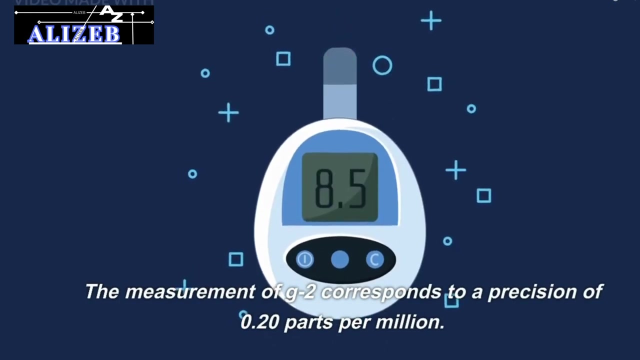 G2 equals 0.00233184110 plus 0.000000000043, STAT plus 0.000000000019, SIST. Advertisement: The measurement of G2 corresponds to a precision of 0.20 parts per million. The Muon G2 collaboration describes: 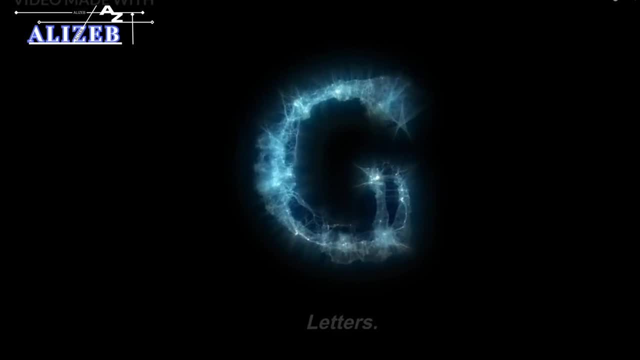 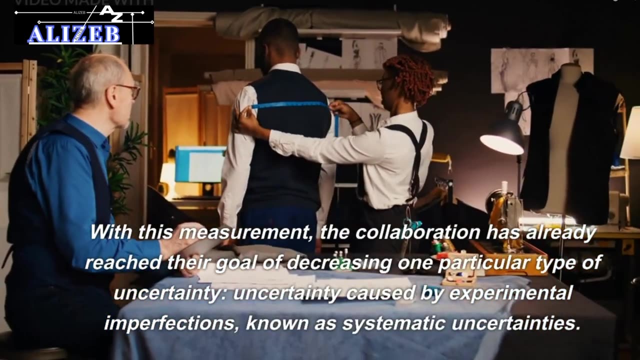 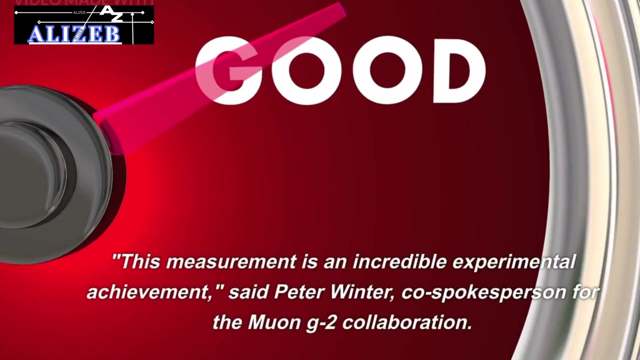 the result in a paper that they submitted today to Physical Review Letters. With this measurement, the collaboration has already reached their goal of decreasing one particular type of uncertainty, Uncertainty caused by experimental imperfections, known as systematic uncertainties. This measurement is an incredible experimental achievement, said Peter Winter. 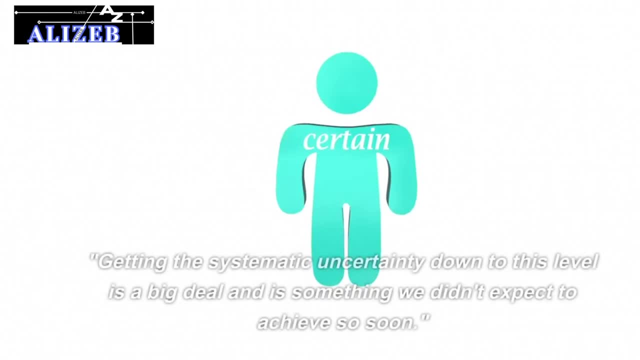 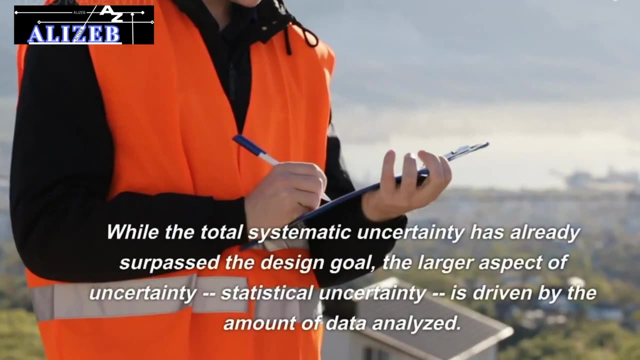 county spokesperson for the Muon G2 collaboration. Getting the systematic uncertainty down to this level is a big deal and is something we didn't expect to achieve so soon. While the total systematic uncertainty has already surpassed the design goal, the larger aspect of uncertainty 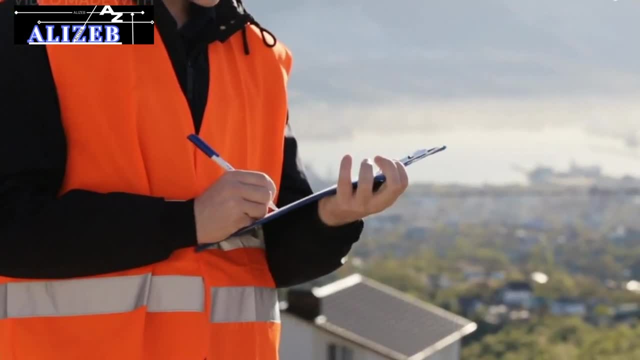 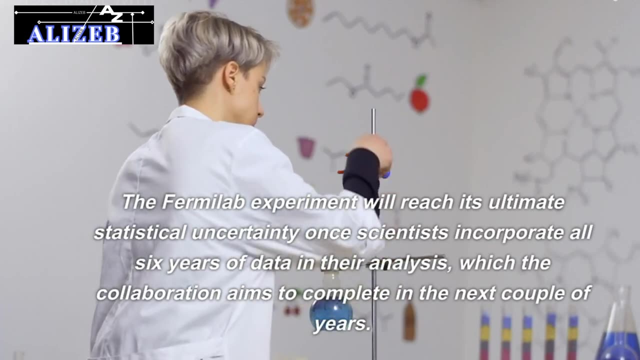 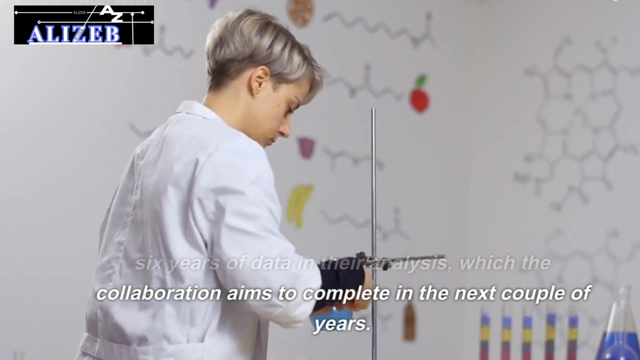 statistical uncertainty is driven by the amount of data analyzed. The result announced today adds an additional two years of data to their first result. The Fermilab experiment will reach its ultimate statistical uncertainty once scientists incorporate all six years of data in their analysis, which the collaboration aims to complete in the next couple of years. To make the measurement 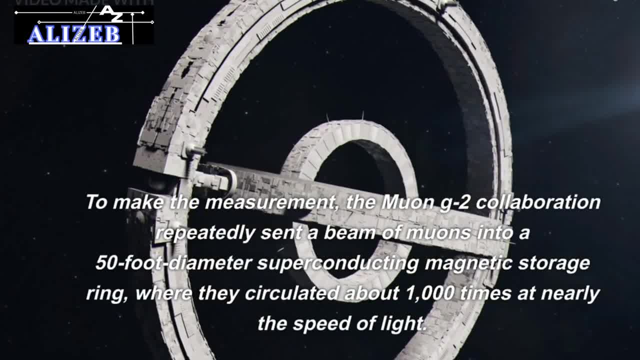 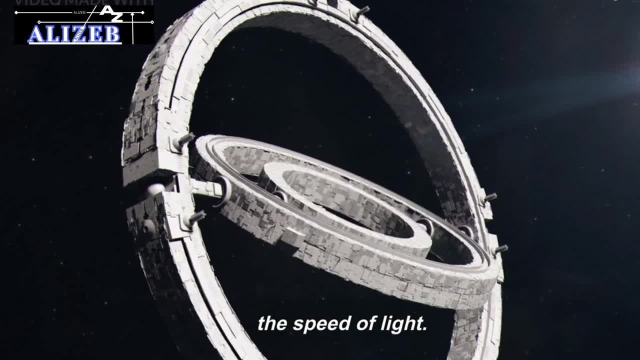 the Muon G2 collaboration repeatedly sent a beam of light to the muon G2 collaboration muons into a 50-foot diameter superconducting magnetic storage ring where they circulated about 1,000 times at nearly the speed of light Detectors lining the ring allowed scientists to 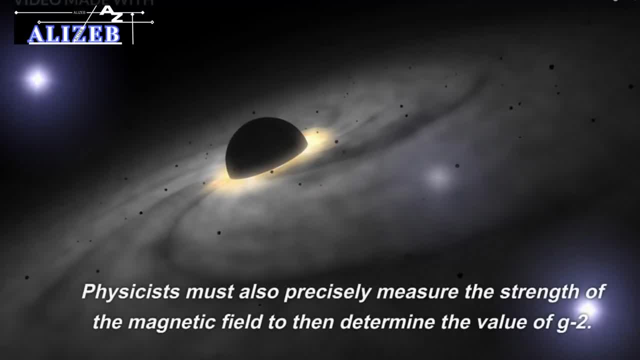 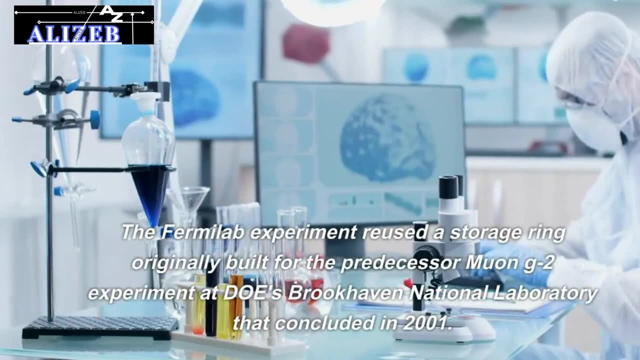 determine how rapidly the muons were precessing. Physicists must also precisely measure the strength of the magnetic field to then determine the value of G2.. The Fermilab experiment reused a storage ring originally built for the predecessor muon G2 experiment at Does, Brookhaven National. 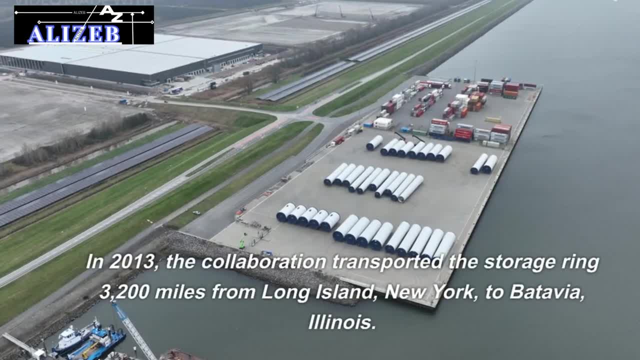 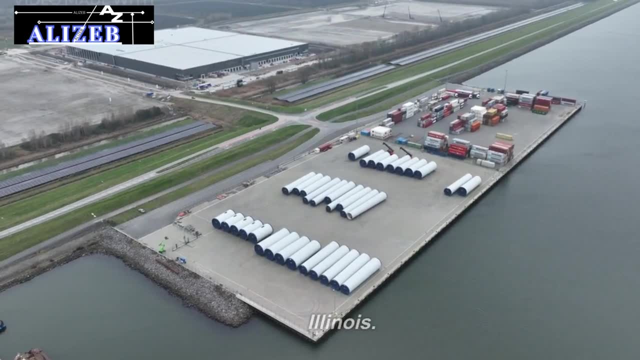 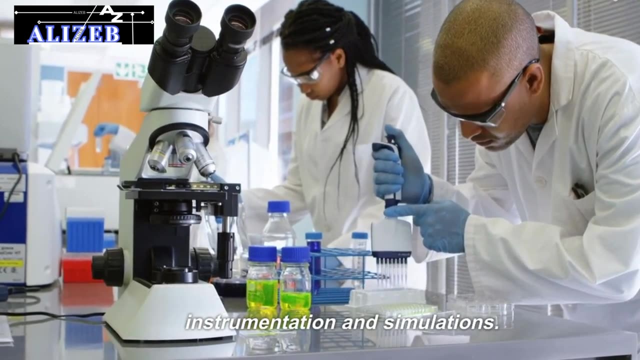 Laboratory that concluded in 2001.. In 2013,, the collaboration transported the storage ring 3,200 miles from Long Island, New York, to Batavia, Illinois. Over the next four years, the collaboration assembled the experiment with improved techniques, instrumentation and simulations. The main goal of 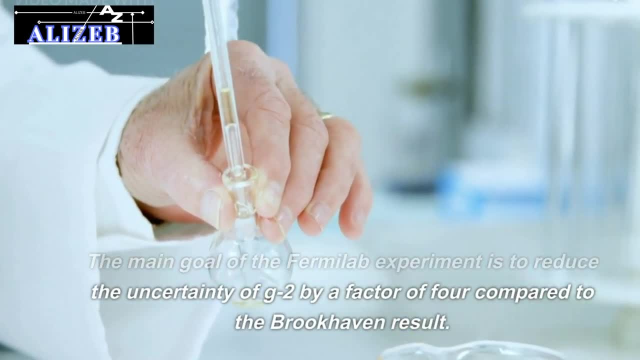 the Fermilab experiment is to reduce the uncertainty of G2 by a factor of four compared to the Brookhaven result Advertisement. Our new measurement is very exciting because it is a very new experiment. It is a very new experiment. It is a very new experiment. 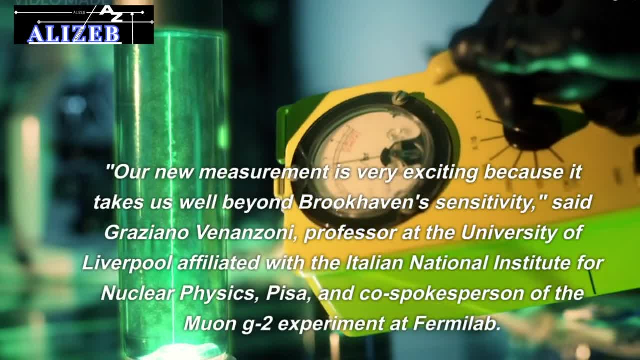 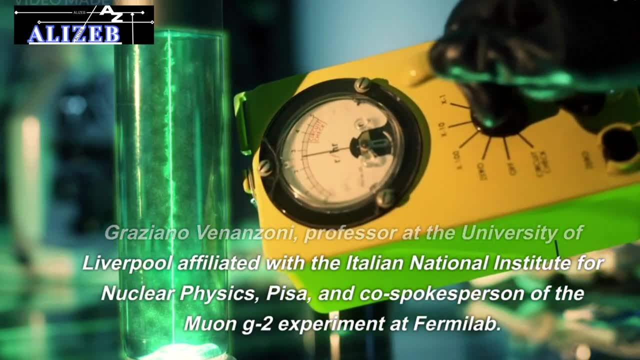 Because it takes us well beyond Brookhaven's sensitivity, said Graziano Bonanzoni, professor at the University of Liverpool, affiliated with the Italian National Institute for Nuclear Physics, PISA, and co-spokesperson of the muon G2 experiment at Fermilab. In addition to the 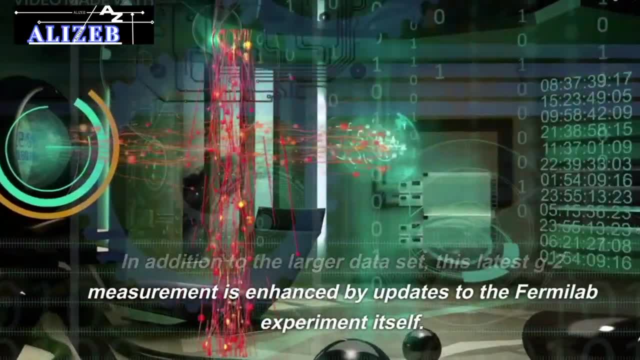 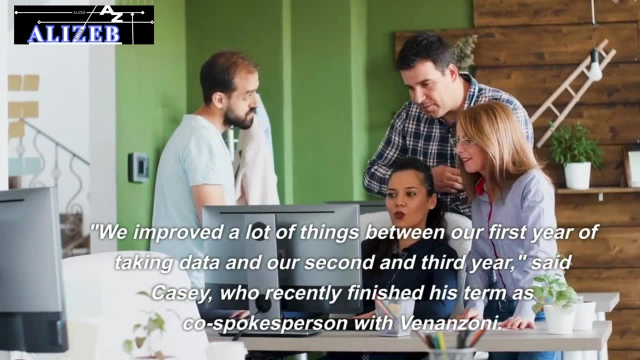 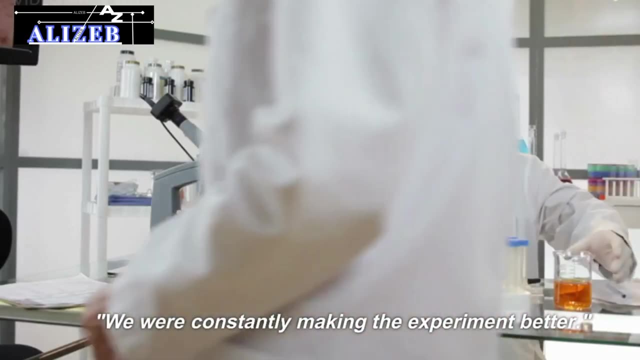 larger data set. this latest G2 measurement is enhanced by updates to the Fermilab experiment itself. We improved a lot of things between our first year of taking data and our second and third year, said Casey, who recently finished his term as co-spokesperson with Bonanzoni. We were constantly making the experiment better. 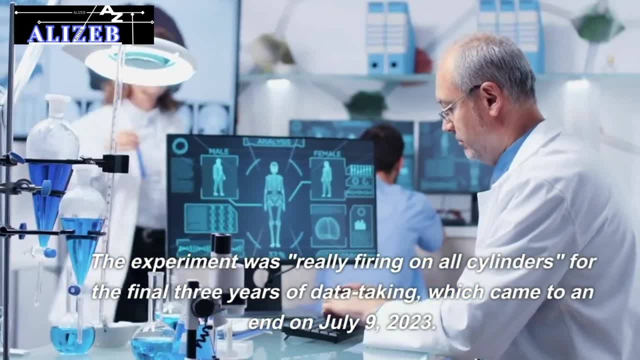 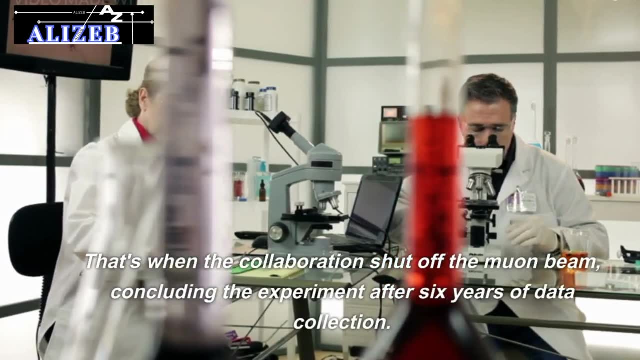 The experiment was really firing on all cylinders for the final three years of data taking, which came to an end on July 9, 2023.. That's when the collaboration shut off the muon beam, concluding the experiment. after six years of data collection, They reached the goal of collecting a. 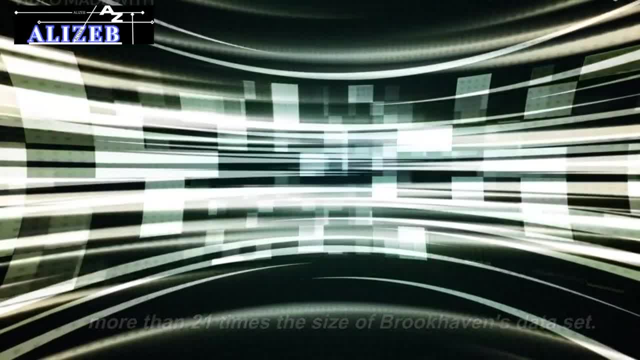 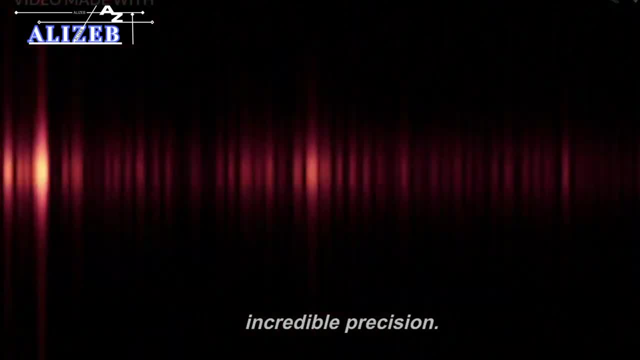 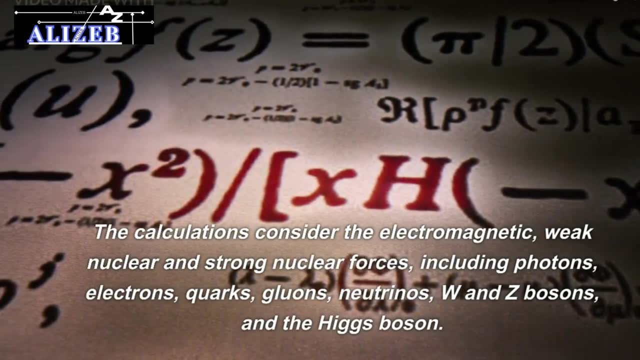 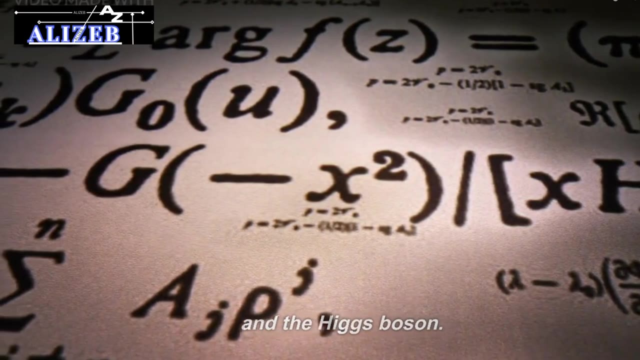 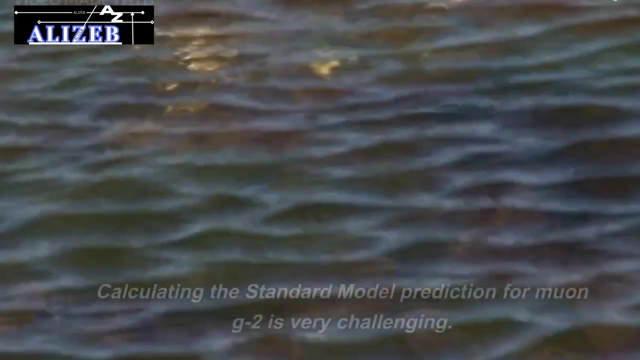 data set that is more than 21 times the size of Brookhaven's data set. Physicists can calculate the effects of the known standard model. If the standard model is correct, this ultra-precise prediction should match the experimental measurement. Calculating the standard model prediction for muon G2 is very challenging. 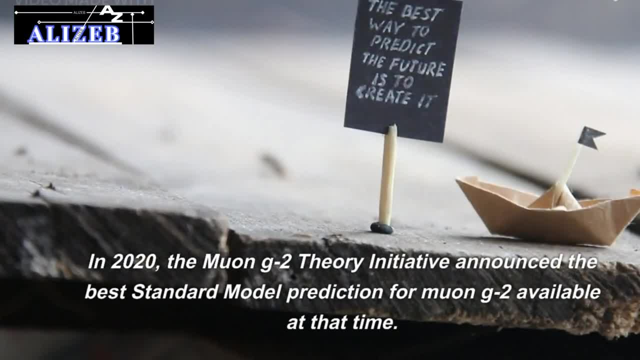 In 2020, we will be able to calculate the effects of the new muon G2 experiment. We will be able to calculate the effects of the new muon G2 experiment. We will be able to calculate the effects of the muon G2 theory initiative. announced the best standard model prediction for muon G2 available. 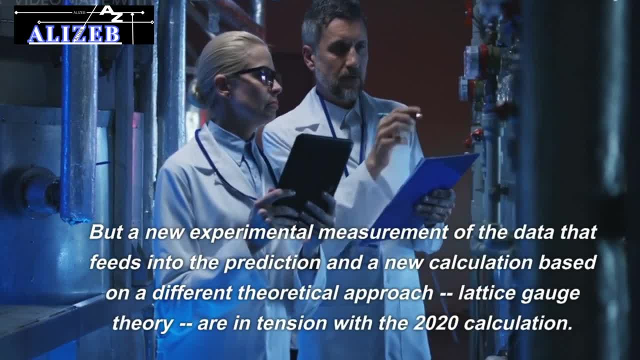 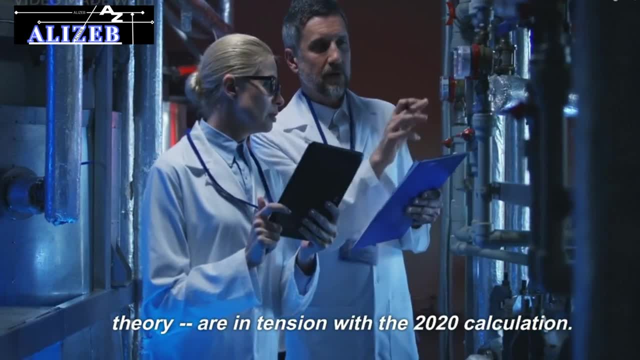 at that time, But a new experimental measurement of the data that feeds into the prediction and a new calculation based on a different theoretical approach. lattice gauge theory are in tension with the 2020 calculation. Scientists of the muon G2 theory initiative aim to have a new, improved 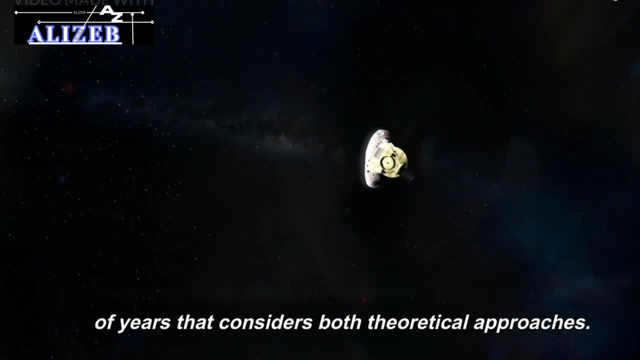 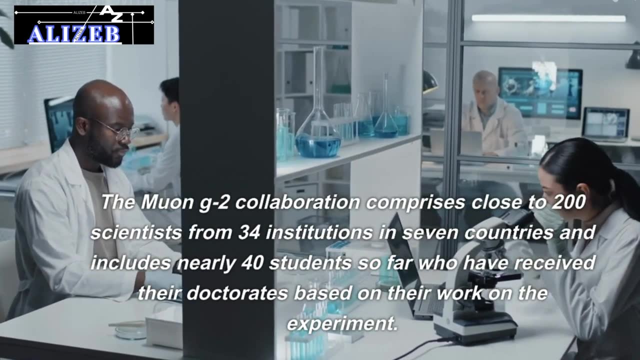 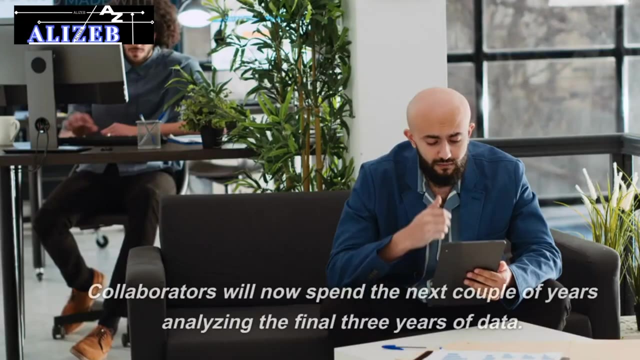 prediction available in the next couple of years that considers both theoretical approaches. The muon G2 collaboration comprises close to two 200 scientists from 34 institutions in seven countries and includes nearly 40 students so far who have received their doctorates based on their work on the experiment. Collaborators will now 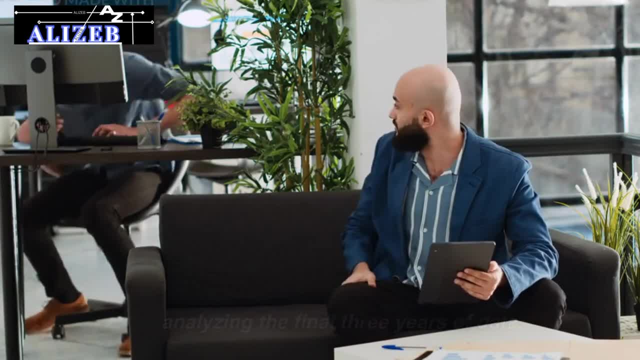 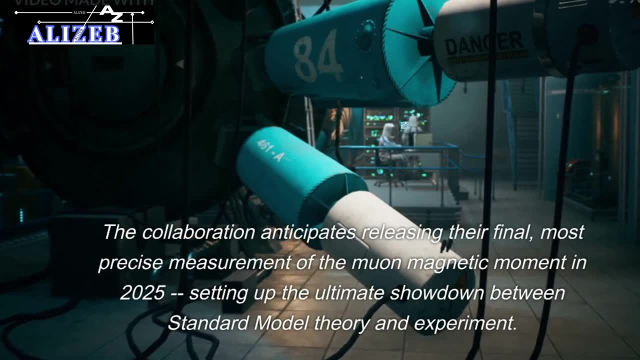 spend the next couple of years analyzing the final three years of data. We expect another factor of two in precision when we finish, said Venanzoni. The collaboration anticipates releasing their final, most precise measurement of the muon magnetic moment in 2025, setting up the ultimate. 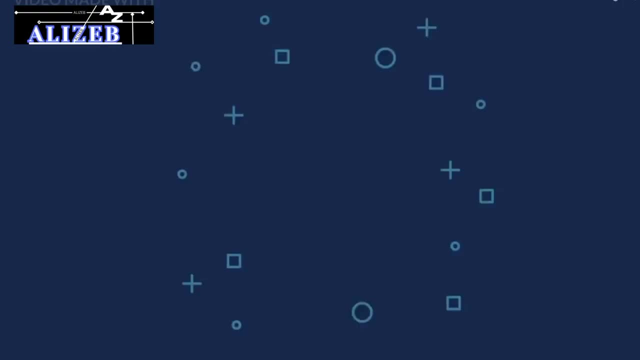 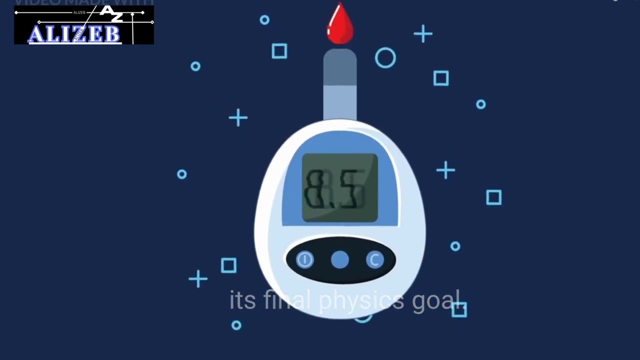 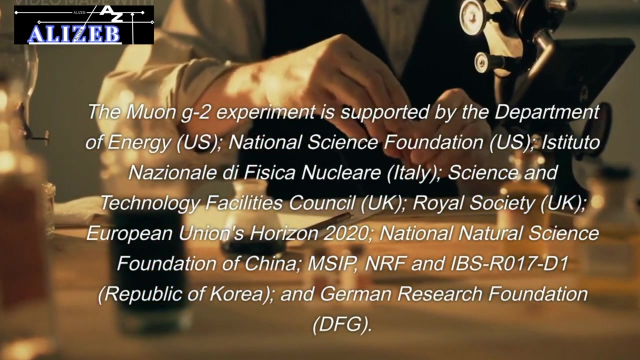 showdown between standard model theory and experiment. Until then, physicists have a new and improved measurement of muon G2 that is a significant step toward its final physics goal. The muon G2 experiment is supported by the Department of Energy, US National Science Foundation, US Istituto Nazionale di Fisica Nucleare, Italy. 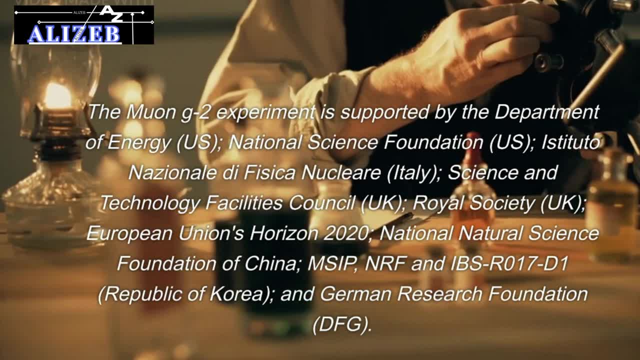 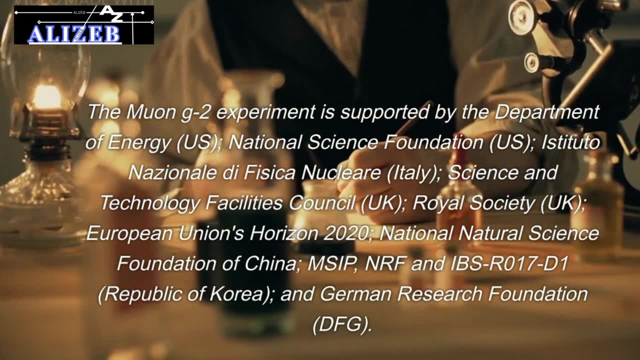 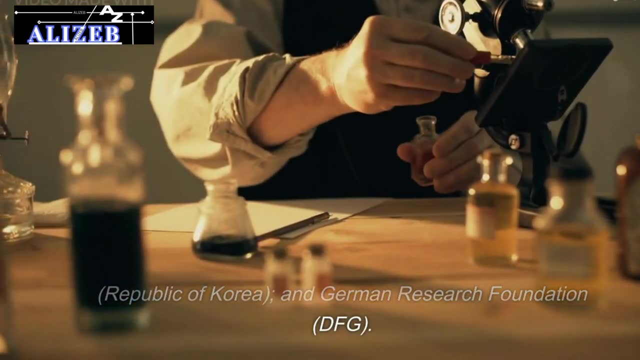 Science and Technology Facilities Council, UK Royal Society, UK. European Union's Horizon 2020,. National Natural Science Foundation of China, MSIP, NRF and IBSR 017-D1,. Republic of Korea and German Research Foundation, DFG. Thanks for watching.